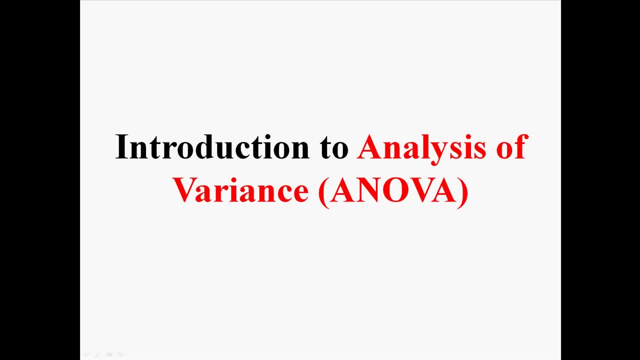 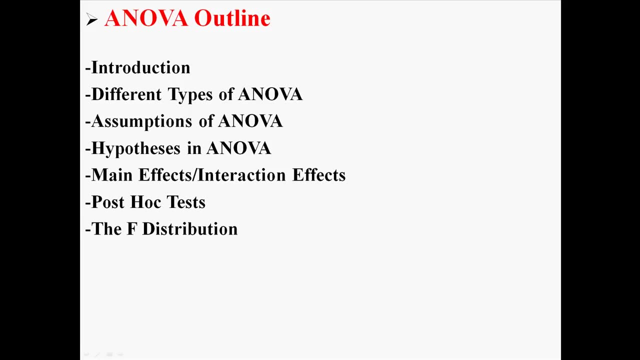 So now I'm going to give you an introduction to analysis of variance, or ANOVA. There won't be any math in this video. I'm just going to talk about what ANOVA is. I'm going to touch on these topics. 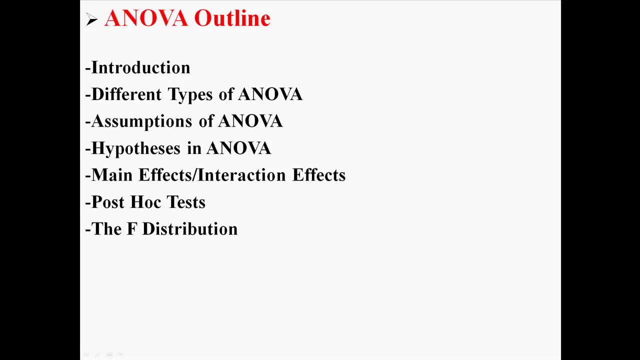 first an introduction to ANOVA, then the different types of ANOVA, the assumptions of ANOVA, how you form hypotheses in ANOVA, what main effects and interaction effects are, what post hoc tests are and what the F-distribution is. 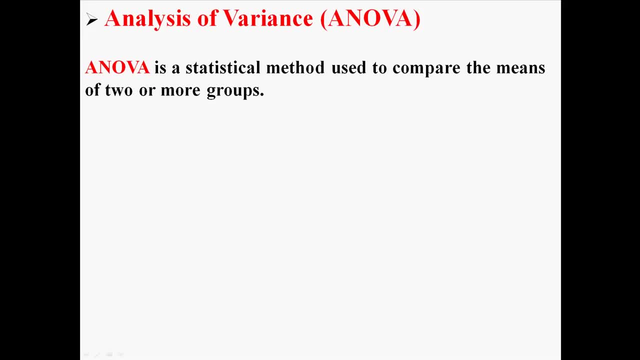 So, first of all, ANOVA. ANOVA is a statistical method used to compare the means of two or more groups. Like before, when we were doing t-tests, we could compare two samples, With ANOVA we can compare three samples, or four samples, or seven samples. we can compare more than two groups. 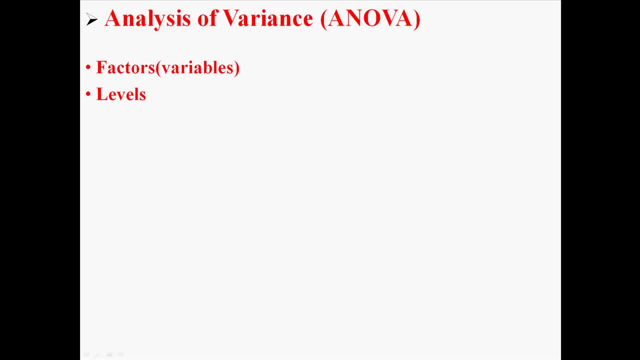 Now in ANOVA you have factors and you have levels. Factors are just your variables. like in one case, gender could be a factor and levels are the levels of those variables. variables like gender could have two levels, male and female, So like here's an example with three: 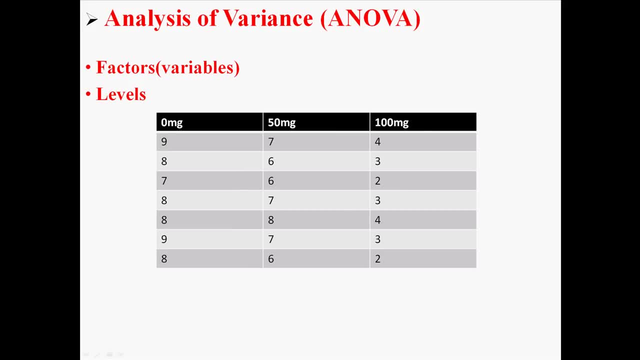 groups: 0 milligram, 50 milligram and 100 milligram. Those are different dosages. So in this case your factor is dosage and your dosage factor has three levels: 0,, 50, and 100.. Now there. 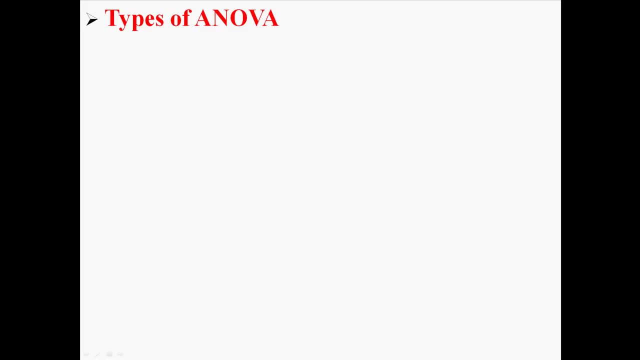 are a few different types of ANOVA and I'm going to show you about three right here. I'm going to show you first the one-way ANOVA. This is an ANOVA that has one factor with at least two levels, and 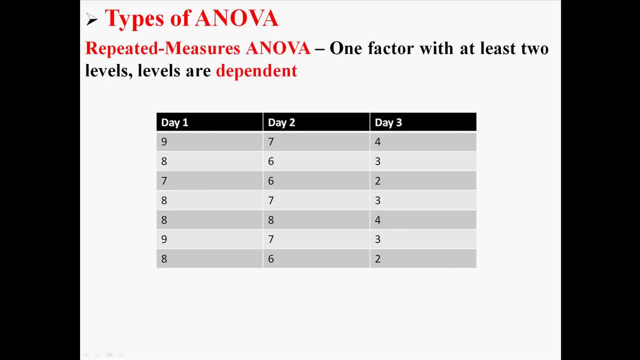 the levels are independent. There's also the repeated measures, ANOVA. This is one factor with at least two levels, but the levels are dependent, Like now you can see, the data has changed. We're measuring the same people day one, day two and day three. It looks almost exactly the same, but 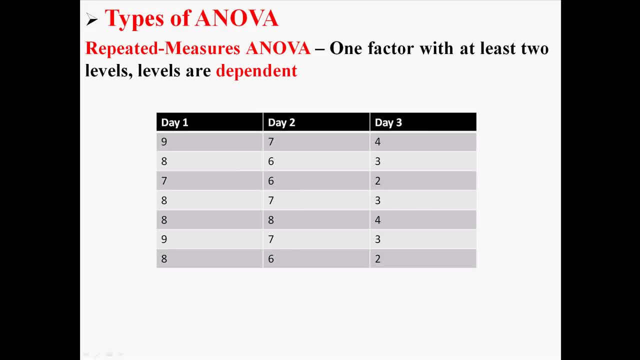 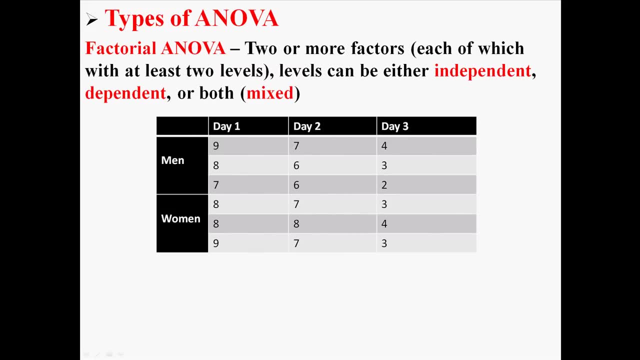 now we're dealing with dependent data, So make sure you know the difference between independent data and dependent data. I actually have a little bit of a problem with that. I'm going to show you a separate lecture on that, if you want to check that out. There's also a factorial ANOVA Now a 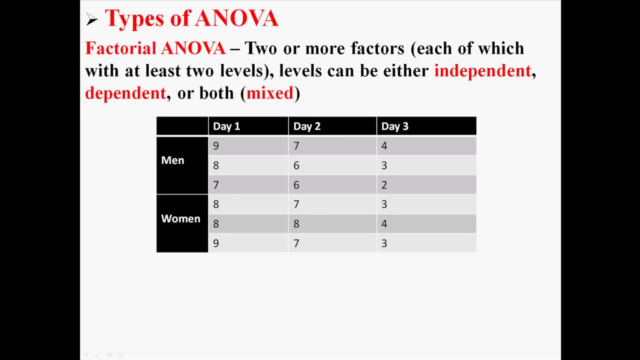 factorial ANOVA has two or more factors, and each of those factors have at least two levels. The levels can be either independent, dependent or both. If they're both, it's called a mixed factorial design. So here's a design that has two variables. One is gender: men and women. 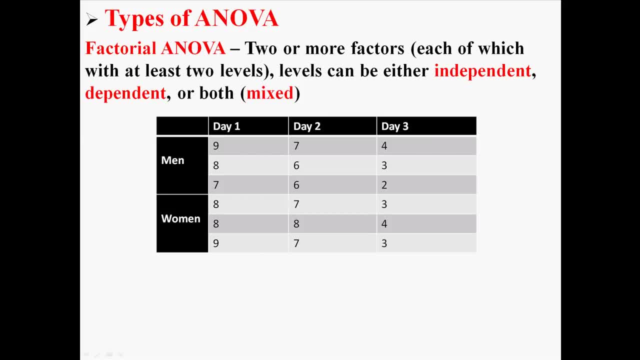 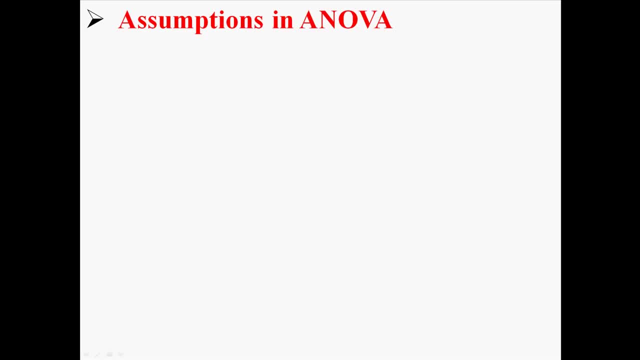 and one is day Day one, day two, day three. So that's two factors. One has two levels and one has three levels. That's a factorial ANOVA. Now ANOVA has a few assumptions. The first assumption is normality. 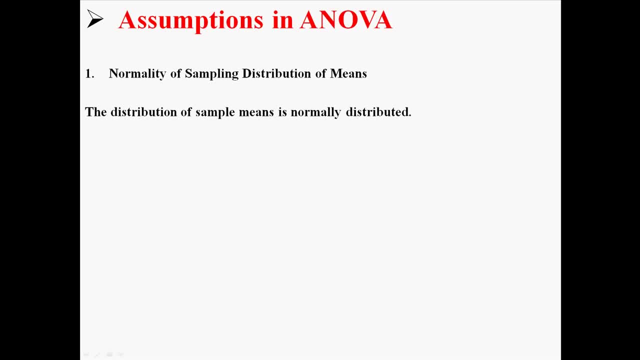 of sampling distribution of means, meaning that the distribution of sample means is normally distributed. We pretty much always assume this is true and it's usually not a problem. The second is independence of errors, That error between cases are independent of one another. The third: 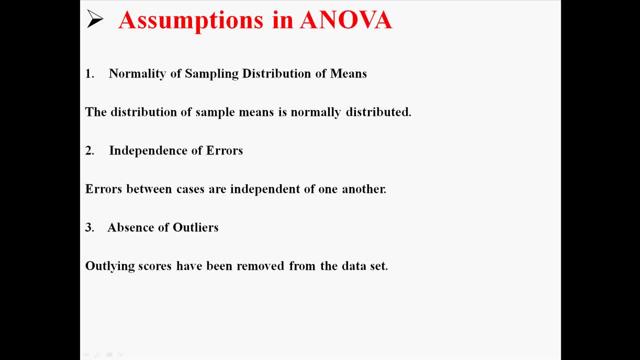 is absence of outliers. Outline scores have to be removed from the data set if you would like to perform an ANOVA. And the fourth is homogeneity of variance, or homogeneity, or however you say it. Population variances in different levels of each independent variable are equal. There's actually a special 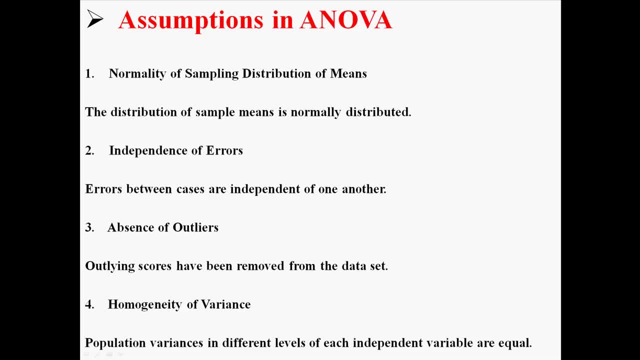 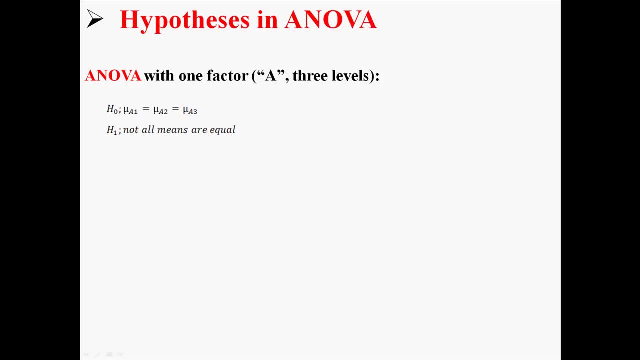 test for that, which I won't do now, but we'll do it when we start doing ANOVAs. Now hypotheses in ANOVA. Imagine you have one factor with three levels. Your null hypothesis is that all three levels are equal to one another. Your alternative is that not all means are. 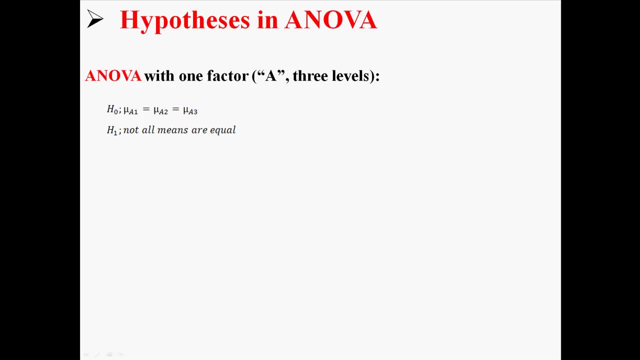 equal. Now you can't write A1 is not equal to A2 is not equal to A3, because that would imply that all three means are different. Maybe only one and two are different, and maybe only one and three are different. so your alternative has to be written, as not all means are equal. When you're dealing, 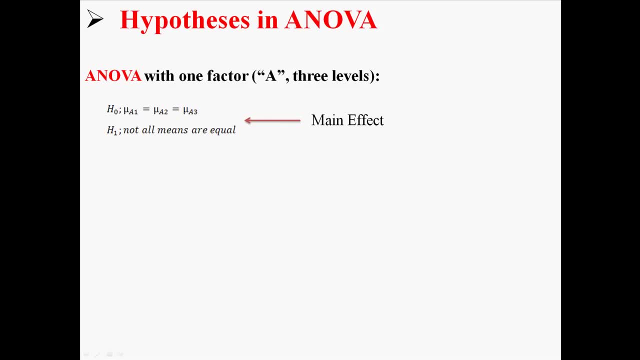 with the effect of one variable. it's called a main effect. But here imagine we have an ANOVA with two factors, A and B- You would have three different sets of hypotheses. You'd have one for A, one for B and one for the combination or the interaction of A and B. And if you had 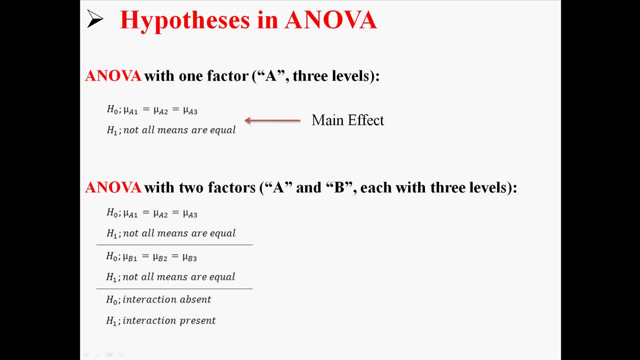 three factors, you'd have even more things going on. So here you have the main effect of A and the main effect of B, and you can also test for the interaction of A and B, which would be structured just like that, The null being, the interaction is absent and the alternative. 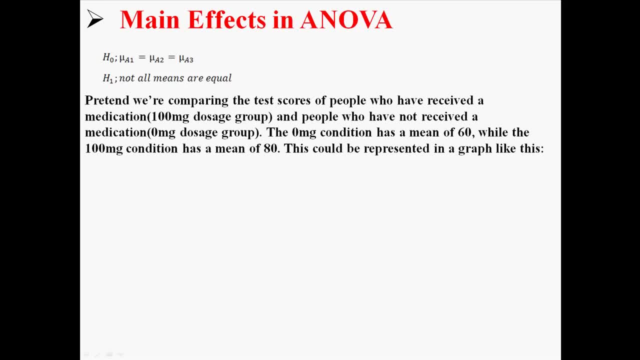 being that the interaction is present. So let me talk a little bit more about that. First of all, main effects. Pretend we're comparing the test scores of people who have received a medication in the 100 mg dosage group and people who have not received the medication. 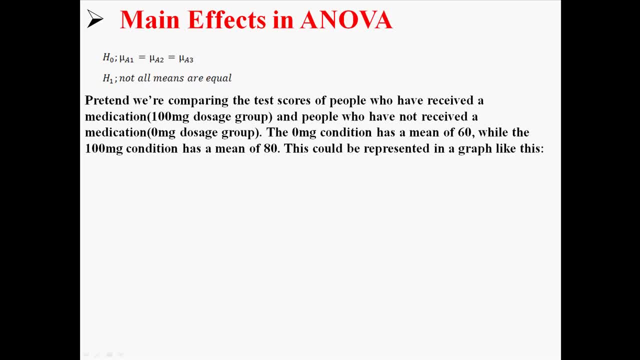 in the 0 mg dosage group. The 0 mg condition has a mean of 60, while the 100 mg condition has a mean of 80.. This could be represented in a graph like this. This would be a main effect: The first group has a mean of 60 and the second group has a mean of 80.. This is 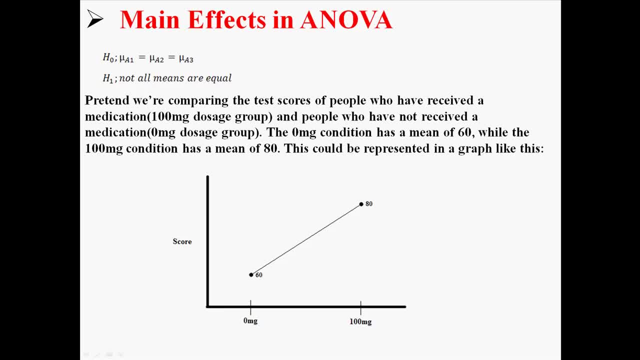 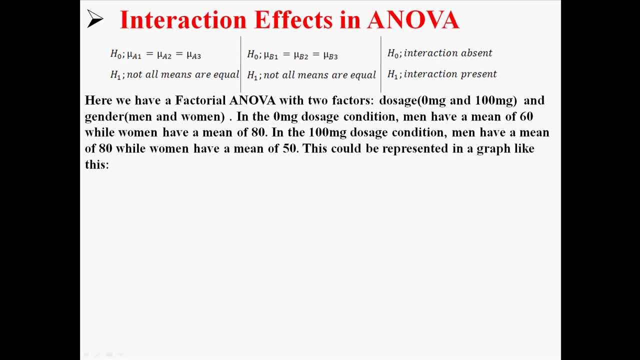 how you could draw it in a graph, And I'm doing it like this because it's a more meaningful way of showing an interaction in ANOVA. So here's an interaction. Let's say we have a factorial ANOVA with two factors. We have 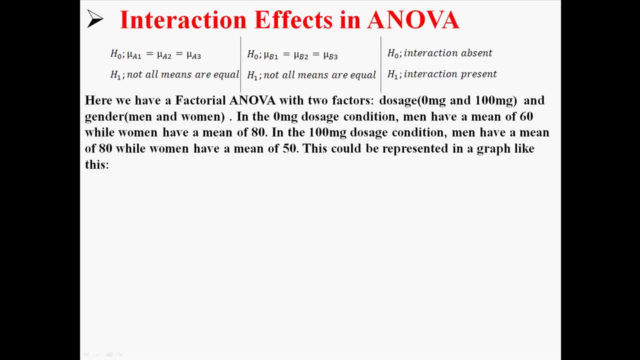 dosage. and now we have gender, men and women. So in the 0 mg dosage condition, men have a mean of 60, while women have a mean of 80.. In the 100 mg dosage condition, men have a mean of 80, while women have a mean of 50.. So now the graph would look something like: 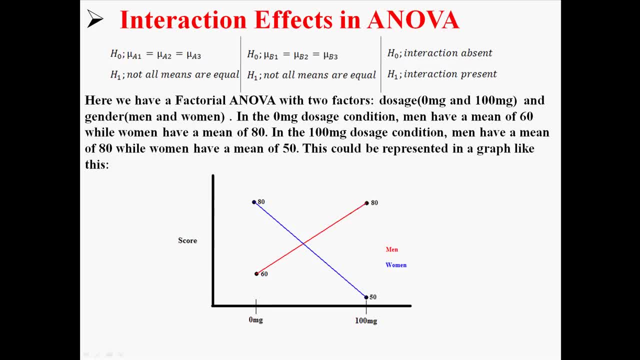 this You can see that the lines for men and women cross. If the lines cross like this, that means you have an interaction effect in your ANOVA. Basically, what an interaction means is that the effect at one level depends on the other level. So, for example, at 0 mg, men are lower than women, but at 100 mg, men are higher than. 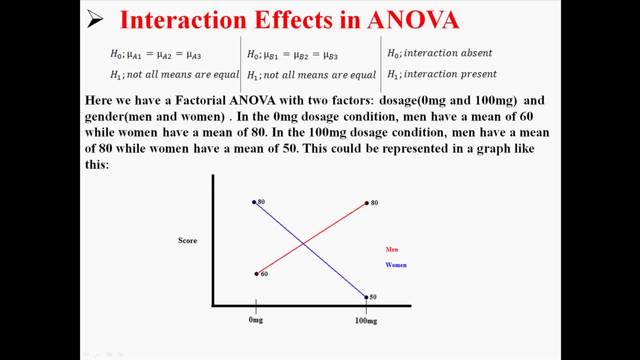 women. So really, the effect of gender depends on what level of dosage you're at, and the effect of dosage depends on what level of gender you're at. The variables have interacted in this way and that's what it means for there to be an interaction effect in your ANOVA. 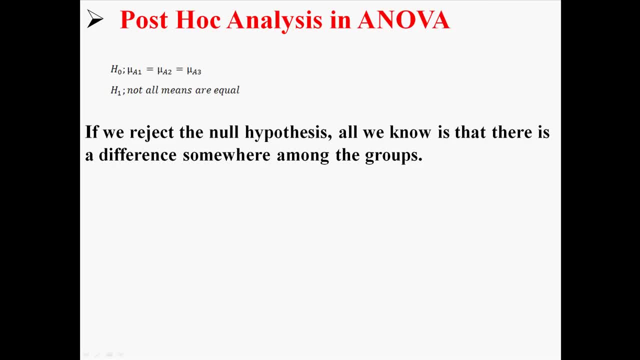 After you do an ANOVA, you might do something called a post hoc analysis Because, remember, if we reject the null hypothesis, all we know is that there is a difference somewhere between our groups. We don't know where that difference is. So additional tests, called post hoc tests,